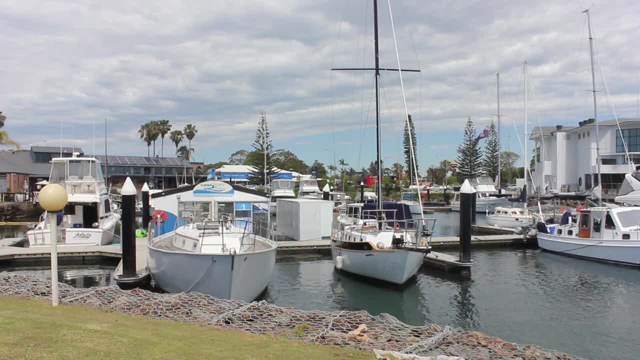 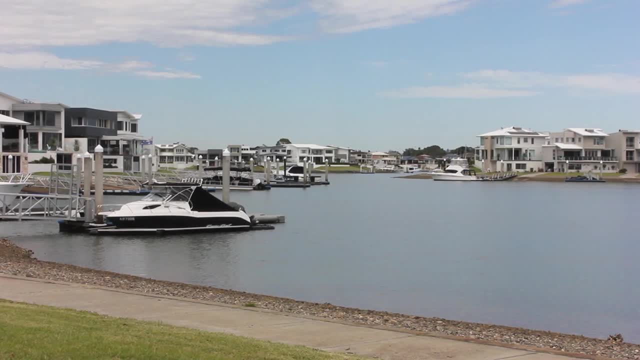 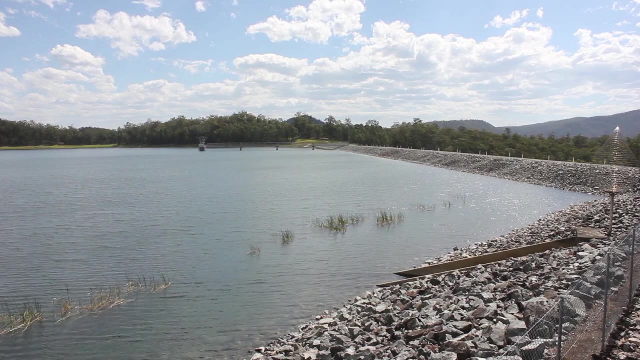 Human activities such as mining, the development of marinas and dredging sand for canal developments all result in sediment being removed from the sea. The damming of rivers also reduces the volume of sediment reaching the coast. All these activities interfere with natural processes such as longshore drift. 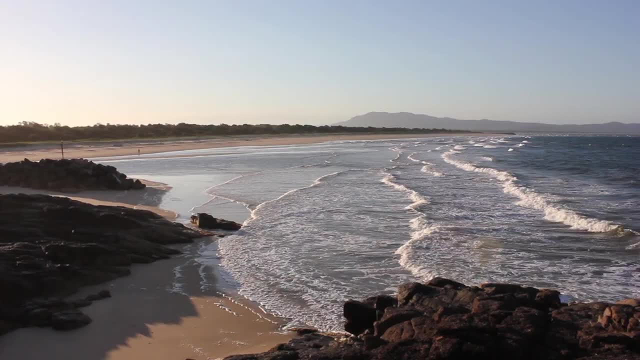 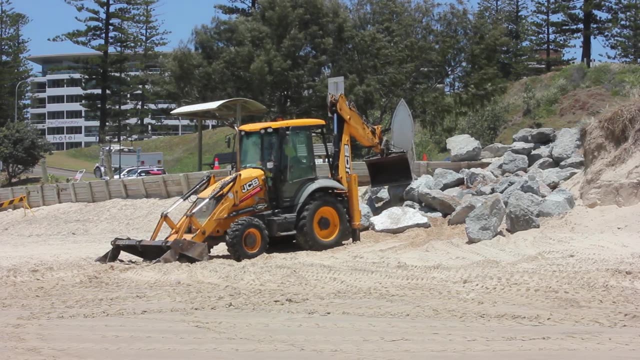 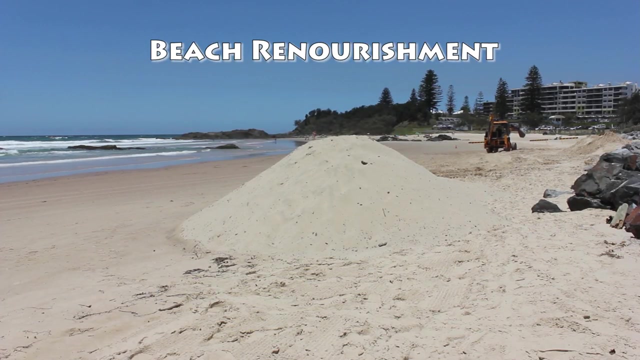 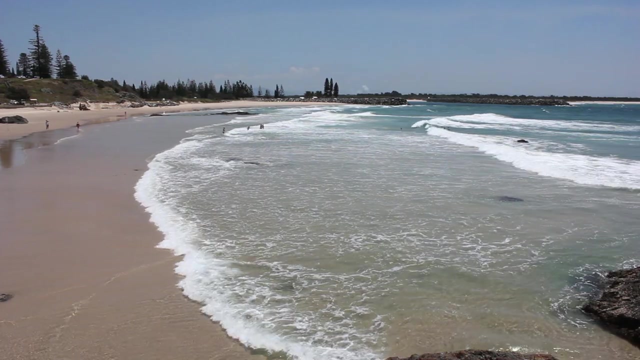 whereby beaches can be deprived of its naturally replenishing sand. Human efforts to deal with coastal erosion include a range of options that have had varying degrees of success in many drawbacks. Beach renourishment is the artificial placement of sand on a beach. Natural processes then spread the new sand along the beach. 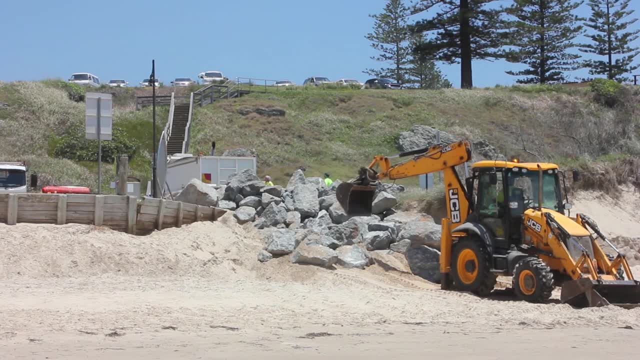 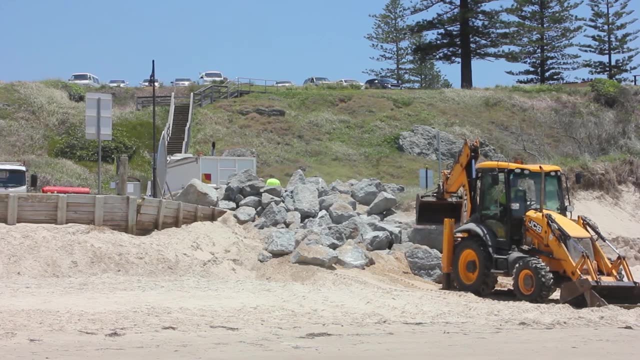 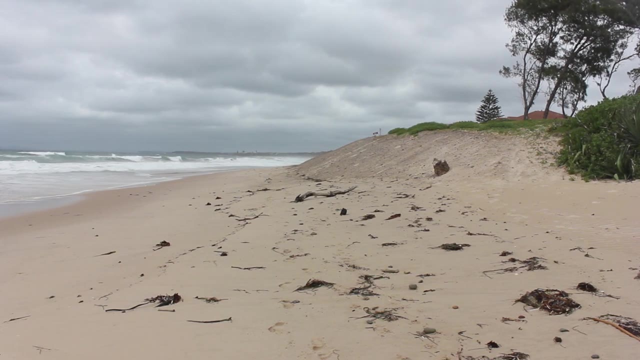 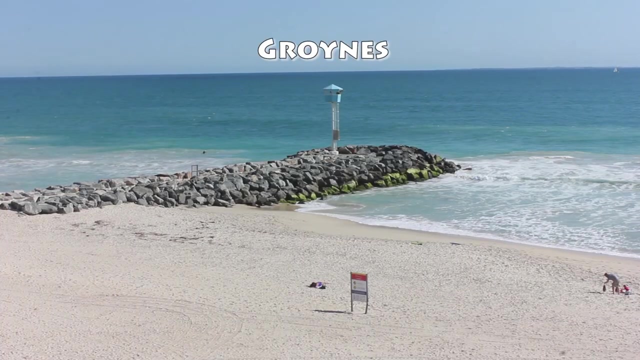 The problem with this solution is that the removal of sand from another beach may have environmental impacts for the beach the sand was sourced from. Another issue is that natural erosion processes mean sand must continually be replaced at the receiving beach, which requires ongoing funding. Another way of preventing the loss of sand from a beach is to construct groins. 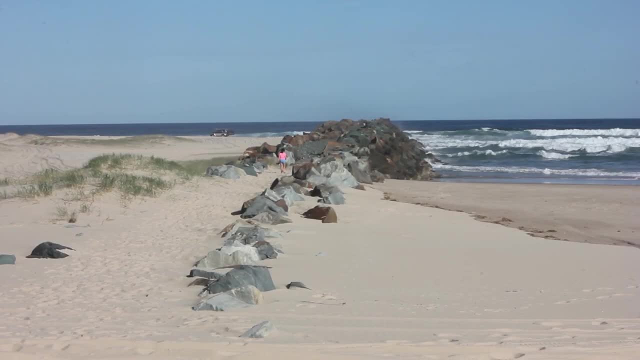 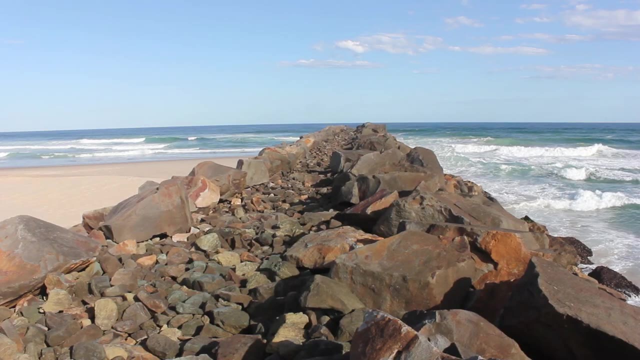 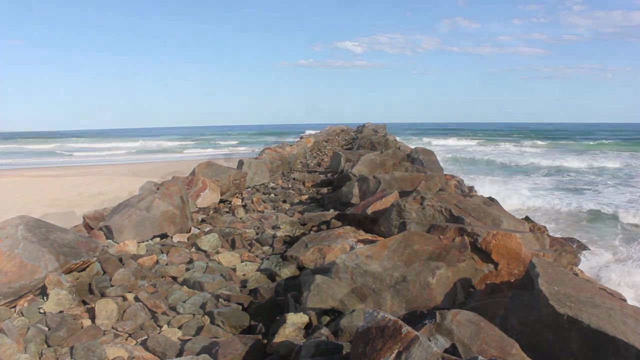 These are structures built, usually extending from the shore out to sea, that are designed to catch the sand that is transported by longshore drift. Groins can be built from materials such as wood, steel, concrete, rubble or sandbags. On the positive side, sand gets trapped. on the up drift side of the groin and a wider 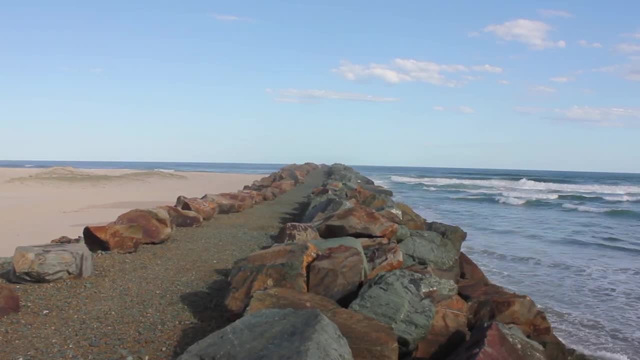 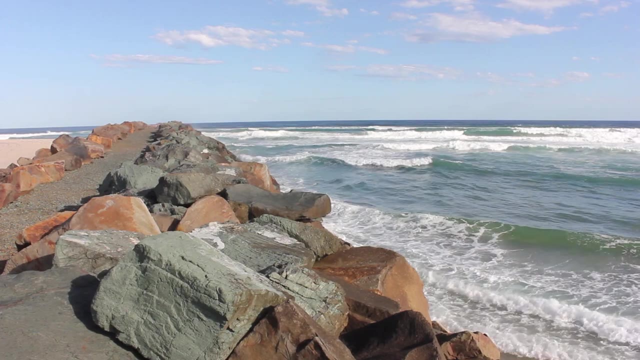 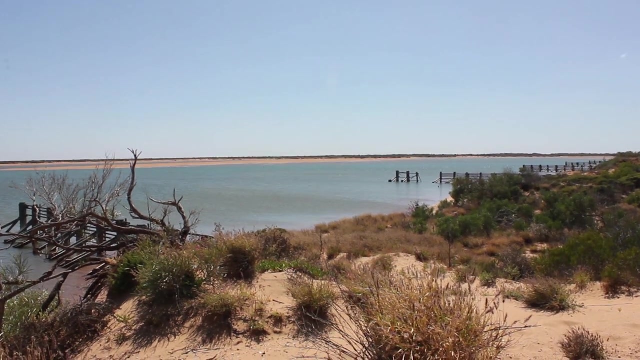 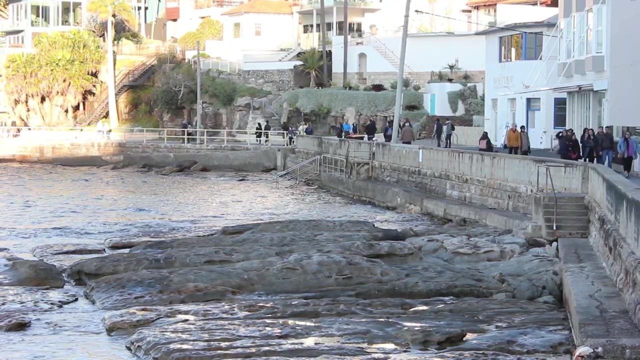 beach is created. However, the effectiveness of groins has some limitations. On the down drift side of the groin, the foreshore is even more susceptible to storm erosion. Groins also fail to prevent sand movement offshore from the groin. A seawall is a structure built to prevent the erosion of dunes and protect buildings. 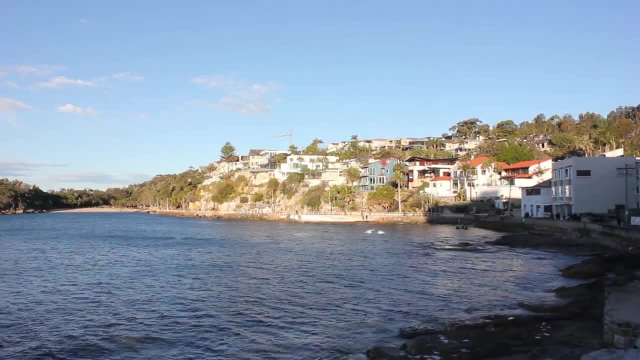 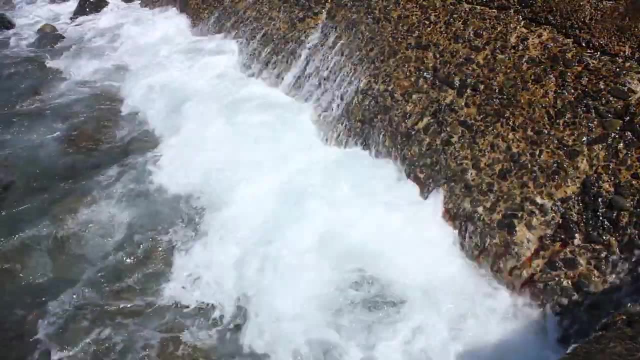 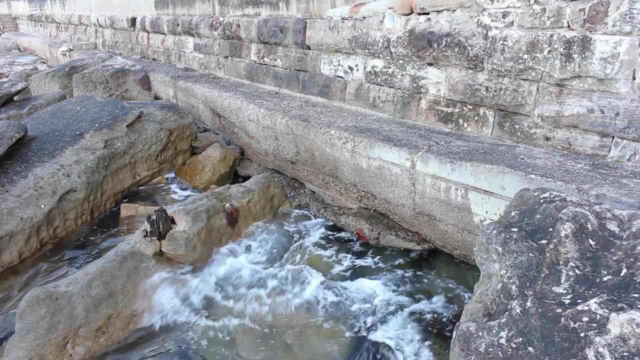 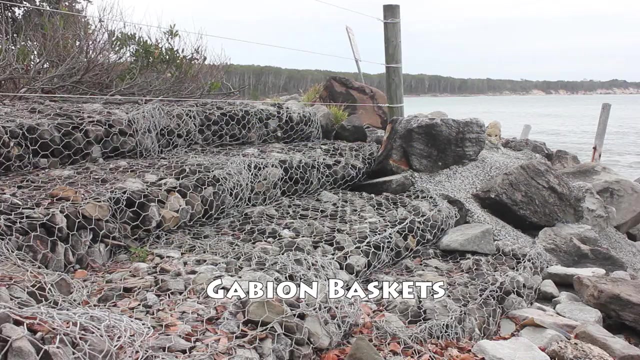 Seawalls are an expensive option And require ongoing maintenance. Waves hitting the wall are reflected. The backwash reflected from the wall drags away sand from the beach. The base of the seawall is eroded over time. Seawalls also destroy the natural look of a beach. 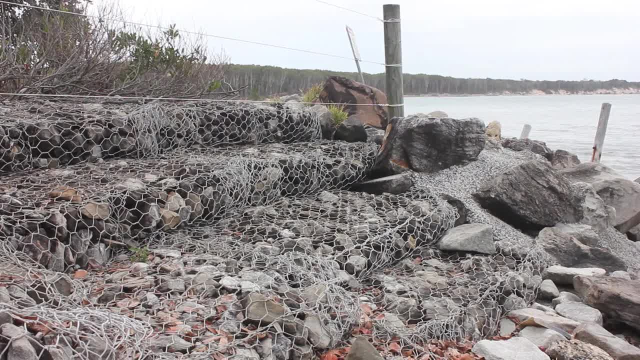 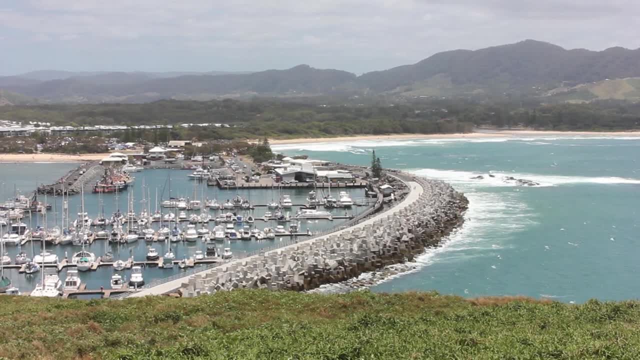 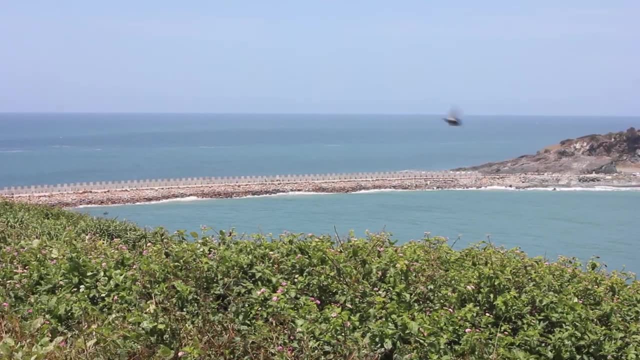 Alternatively, some councils place large rocks and gabion baskets on the beach to try and protect it. Some councils may choose to construct an off shore breakwater. This is a structure parallel to the shore and placed in the water at a depth of about 10 metres. 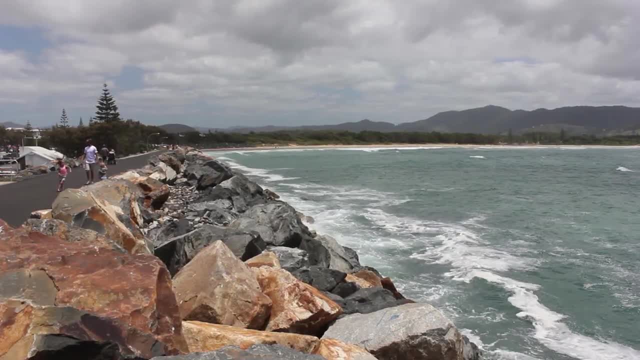 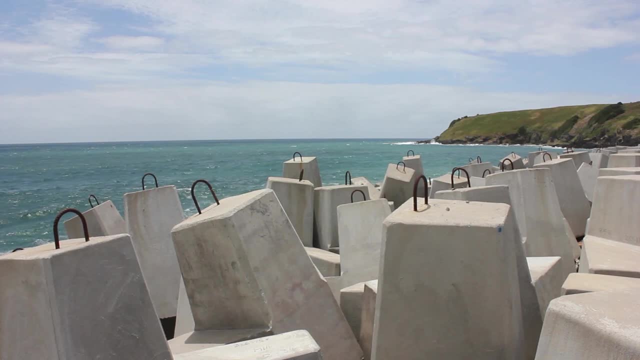 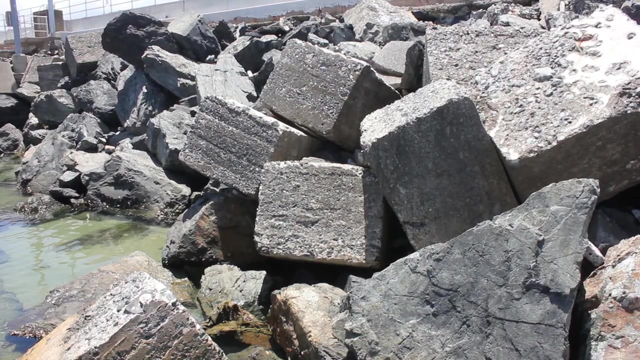 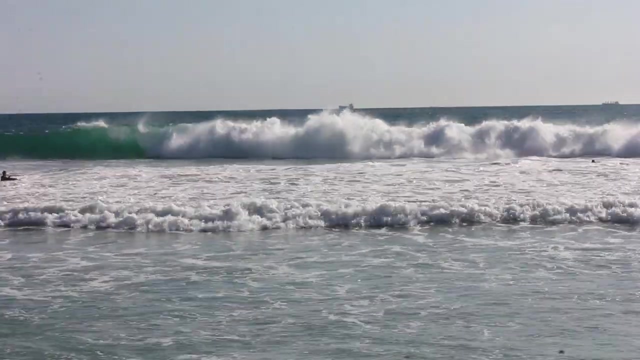 By doing this, waves will break in the deeper water, reducing wave energy and erosion at the beach. The downside of offshore breakwaters is that these structures require many large boulders and can be very expensive. Surfing communities are also opposed to this solution because it destroys the availability of surfable waves. 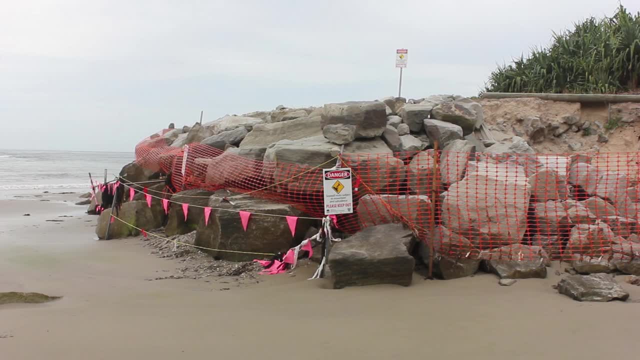 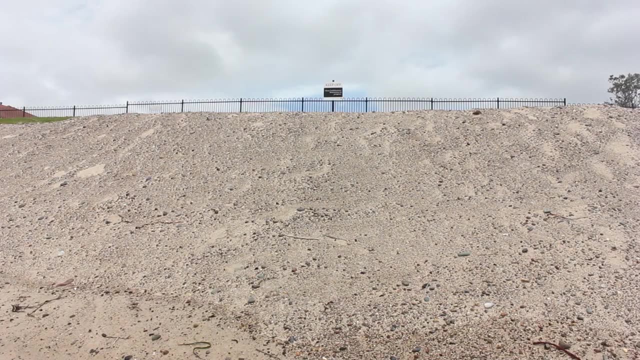 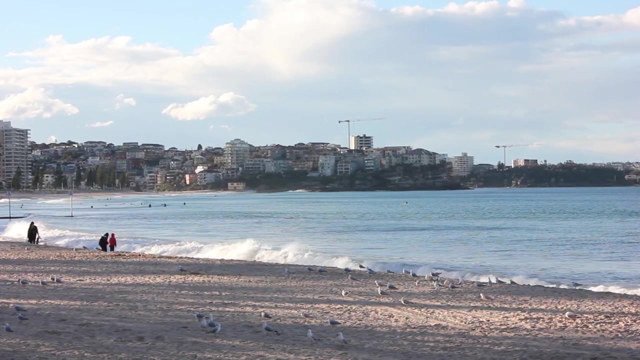 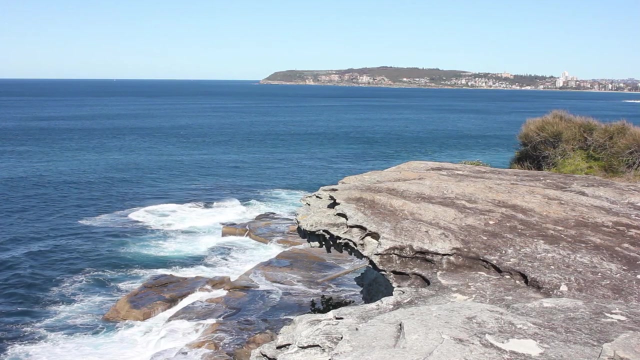 Given the failure of seawalls and other hard structures, new approaches are being taken to coastal management. One of these is a managed retreat from the coastline. A council may buy coastal properties and remove any buildings threatened by erosion. This makes it easier to manage as it allows coastal processes to continue. 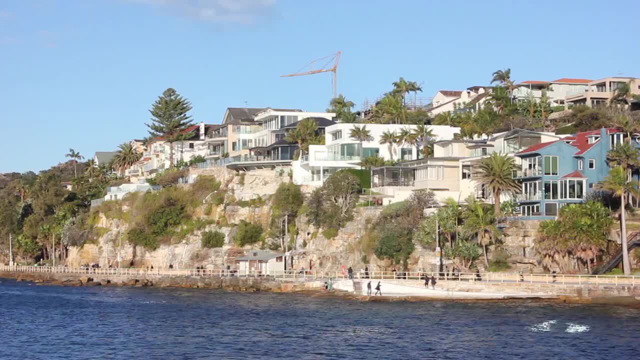 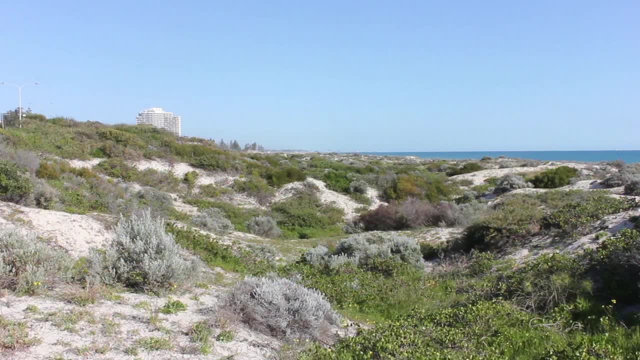 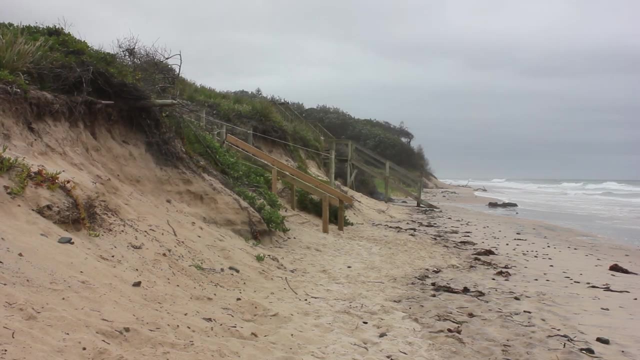 But buying properties is very expensive and it still does not solve the long-term problem of the loss of land to the sea. It is important that people look after sand dunes. They form a natural barrier to wave erosion. They are also home to endangered shorebirds such as the Little Thames. 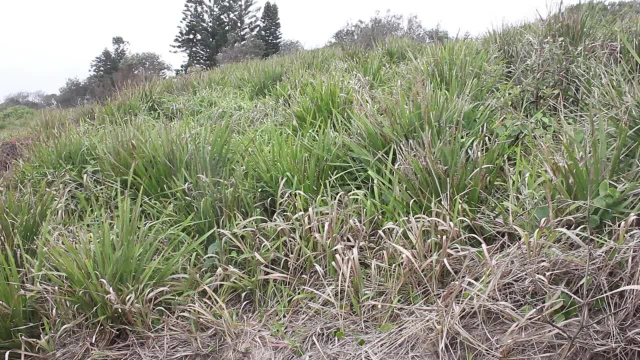 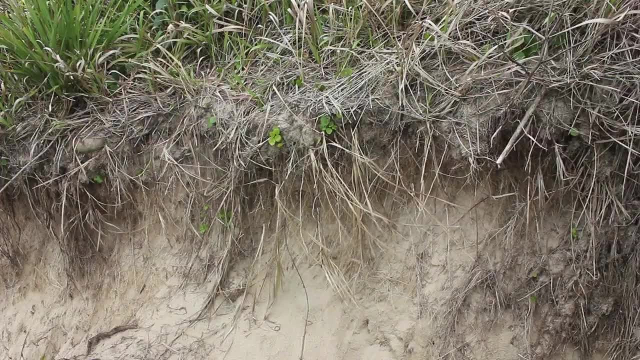 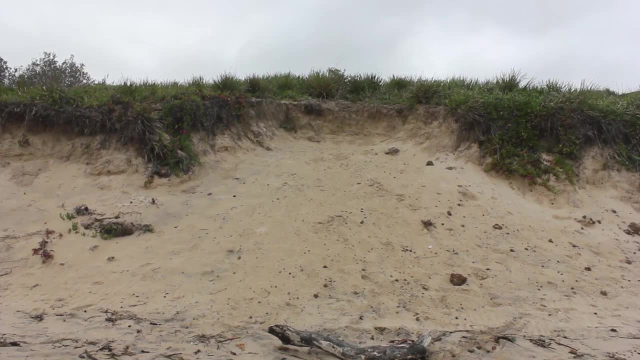 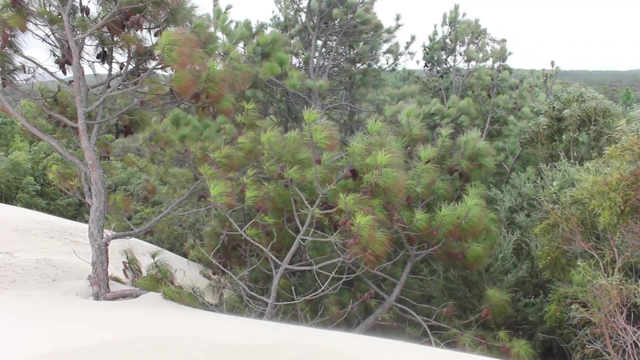 They will turn, but lay their eggs there. Vegetation is essential for stabilising dunes. It is the vegetation that traps the sand and holds it in place. If a vegetation cover gets removed, wind will remove the sand, leaving a blowout. If the natural vegetation cover is removed, dunes can also advance inland. 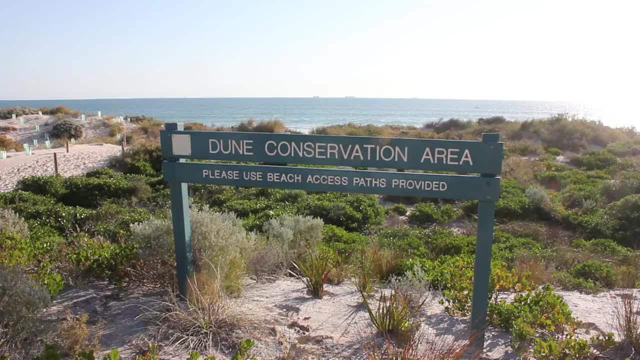 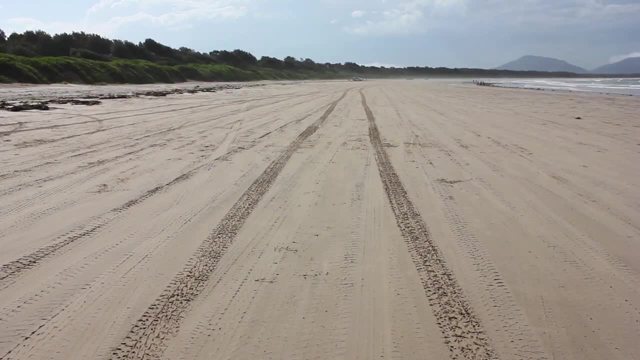 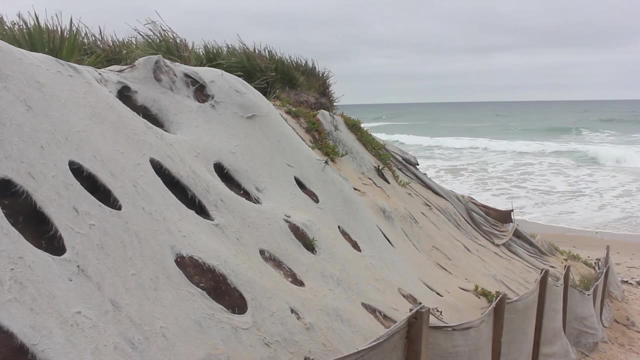 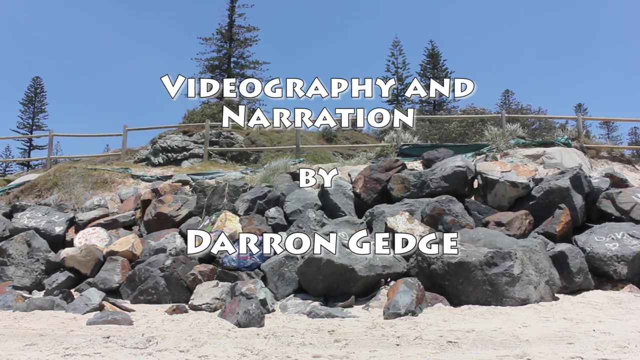 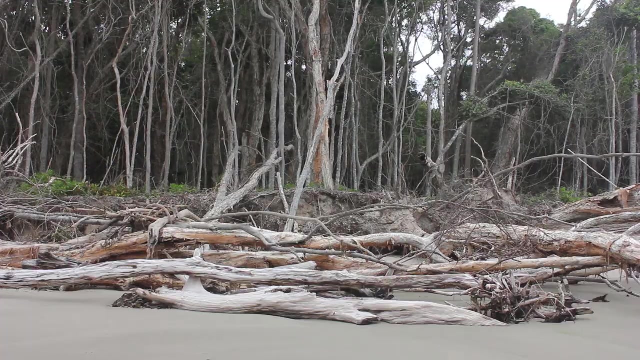 Such as the driving of four-wheel drive vehicles on the beach, walking and fires threaten the vegetation cover of coastal dunes and thereby enhance erosion. Councils have met these challenges by fencing off the dunes and by conducting re-vegetation projects. They have also met the challenges of re-vegetation projects.